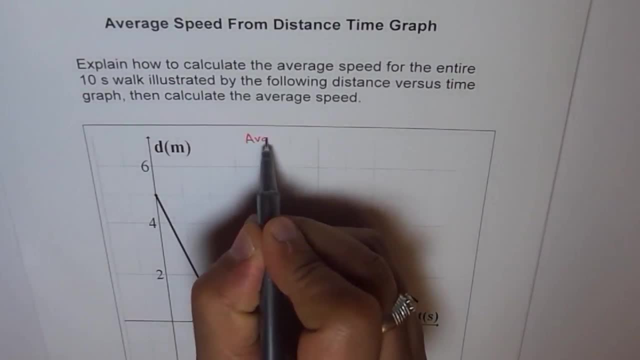 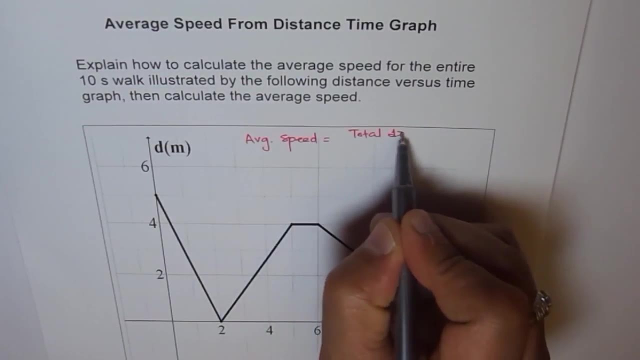 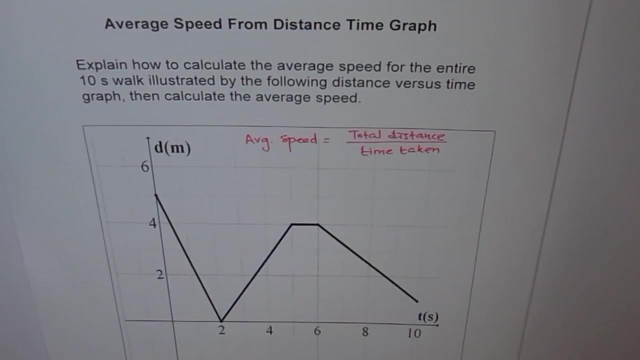 average speed is how much. We say average speed equals total distance over time taken, right? So here we know the time taken is 10 seconds. Now how much is the distance? That is a big question, right? I've seen it looks very simple problem, but many students get it wrong. Now 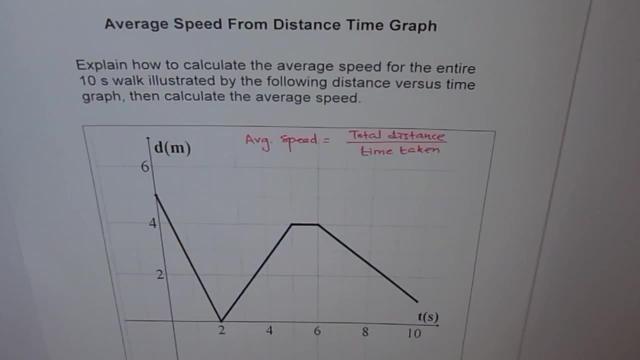 let's understand how to calculate the distance from here. So at zero, what do you think is the distance? The starting distance is five, right? That means a body is actually five units away at starting point And in two seconds it comes to the point from where the distance being measured, right? 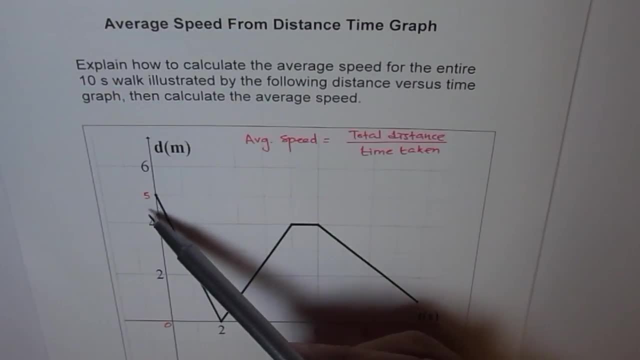 So that means in two seconds. how much distance did we cover? We covered five units, which is meters. So the distance covered in first two seconds here is five meters right, Plus after five meters from two to this unit is five. how much distance is covered So from? 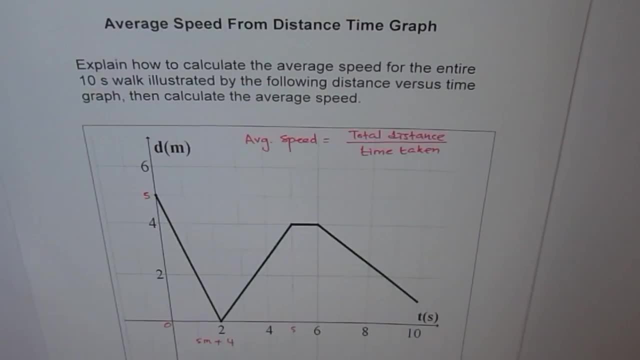 zero, we went to four, So it was plus four right. And then here no distance is covered because the body stayed at four itself. so like stationary right, Zero meters. And then from here to ten seconds distance covered is from four to this is at one right. So four to one is one to three. 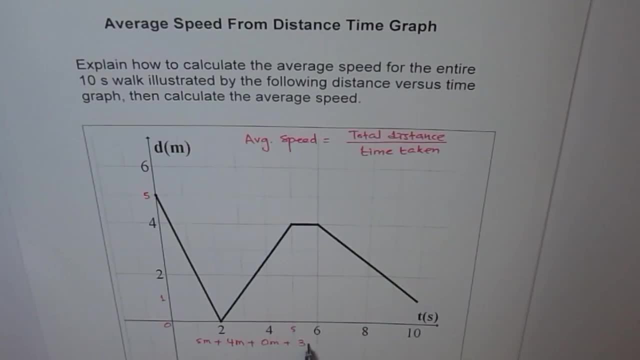 units. So it is just three meters. right, people and students measuring the diagonals right and and adding up the diagonals. no, that is not the distance. it looks like a diagonal, but actually distance is five units. right, you started at five and came down to zero. therefore, the distance in first two seconds is not this: a square plus b. 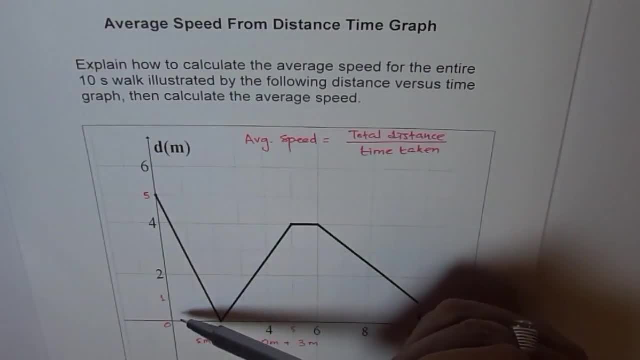 square, square root, not the hypotenuse of this, but it is just five minus zero, right, because distance is always taken positive. if, if it was displacement, then it was a different story. all together, right, if it was displacement, can you tell me what was a net displacement?